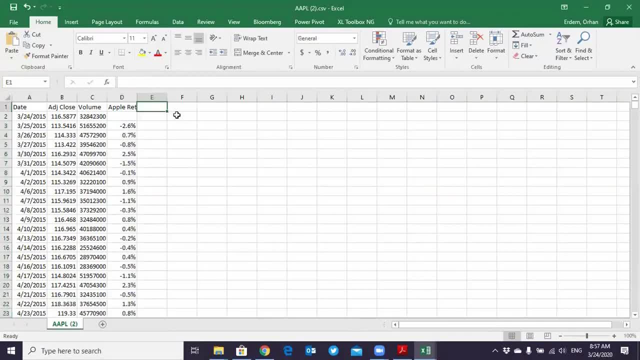 it with the volume directly, or you can also calculate the change in volume here. That will be fine. Let's see how the volume changes from yesterday to today. So this is going to be percentage change of volume. You can do it with the volume itself, fine, but let's just do it with volume change. Let's just like 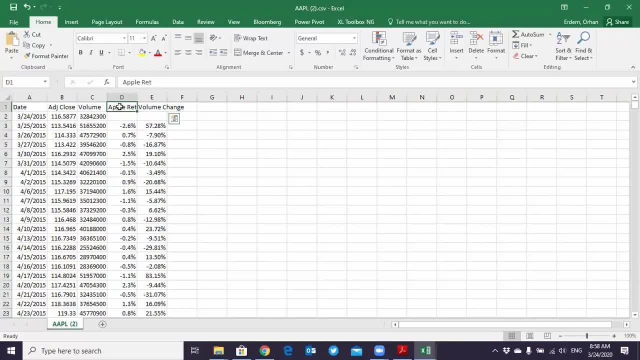 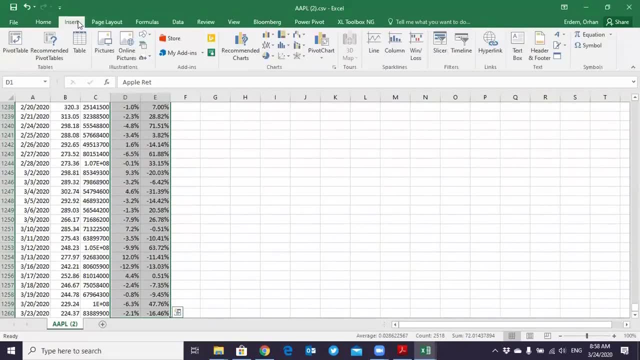 draw them both together. Just select these two things using your mouse, Then drag and drop, or use ctrl shift down arrow to select the whole column. Go to insert. from insert there is line chart here. click line chart and select the very first one here. 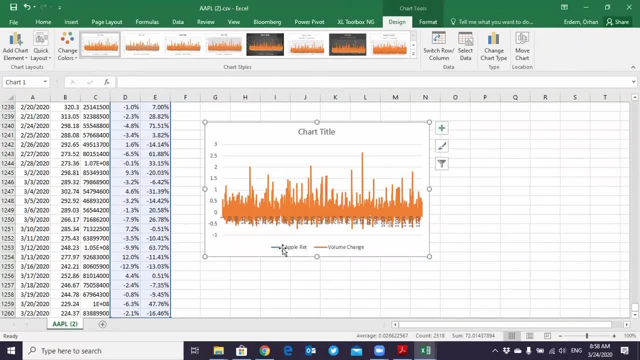 Okay, so in this volume, the blue one is Apple returns and orange one is volume change. but as you can see, the volume change kind of its too much and it can probably hides the Apple returns. What we can do in the dollar chart is to do the chart here forms 강 En Key This few. 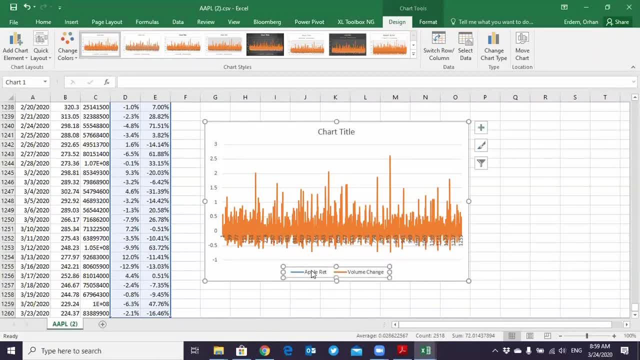 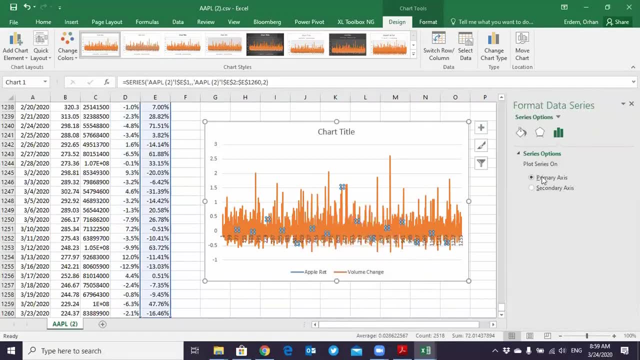 performed as the stock value of Apple in 30 minutes. And then we young people, and then we just do the hedging And then I choose exactly in 80 percent. now지 is right. click on the data, click format data series and change it to secondary. 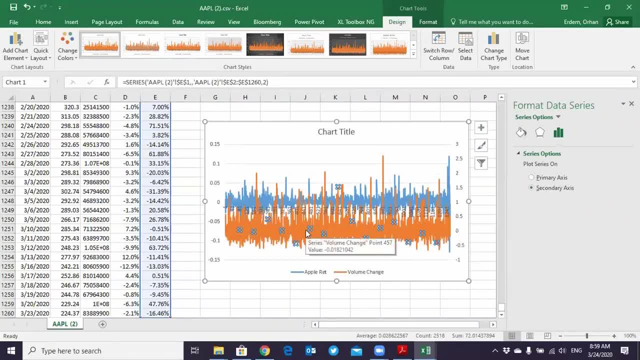 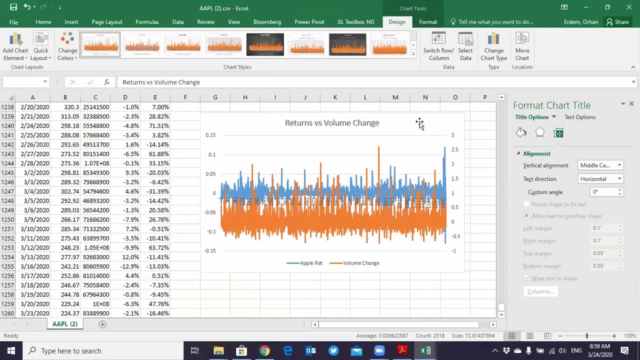 axis so that you can see them both. so right click on the chart and then format data series and secondary axis. so the blue one is Apple return and orange one is volume change. so change the chart like title to returns versus volume change. so one thing we did not do here is on x-axis you see numbers we should. 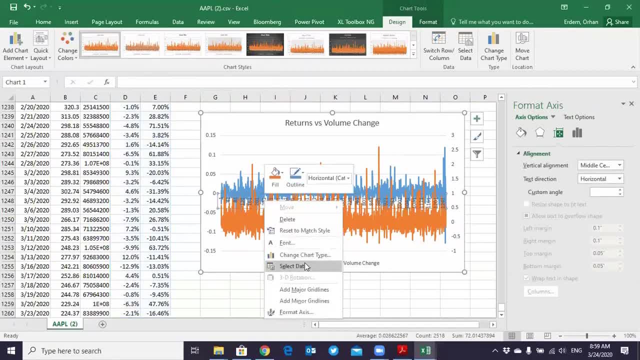 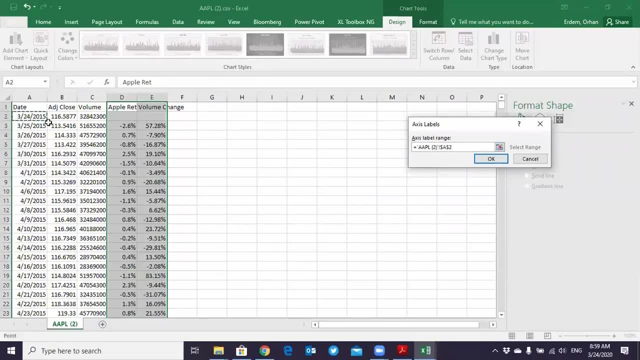 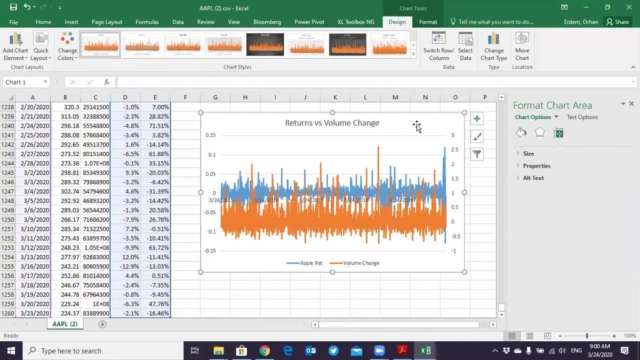 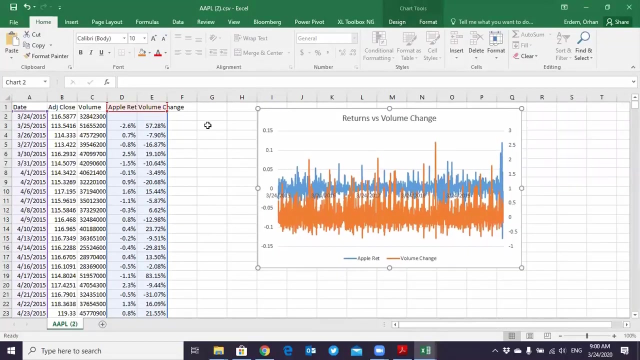 change it to dates. right click on the date, select data code. like you will see any window here. hit edit here and select the dates. okay, so this is going to the dates of x-axis. so now you see your dates. so this is one way of comparing returns with volume change visually. but if you want to have some like concrete or 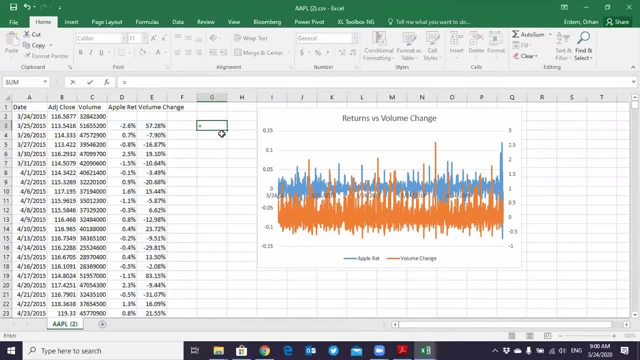 solid number so you can click on any cell and write Corel. so for Corel it's asking two data series, the first one, the second one here. for the first one, choose Apple column okay, and then comma. do the same thing for volume change. so hit the very first cell and then ctrl shift down arrow will. 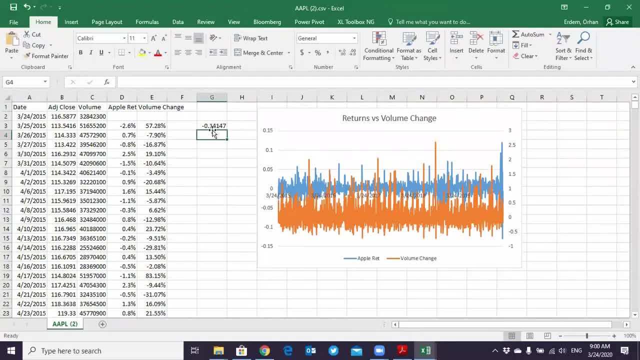 select all and close the parenthesis so you would see some number here. negative 14. so, as you might know, correlation coefficient- this is called correlation coefficient. it shows the relationship between two data series, it is between two data series, it is between two data series and it is between two data series. 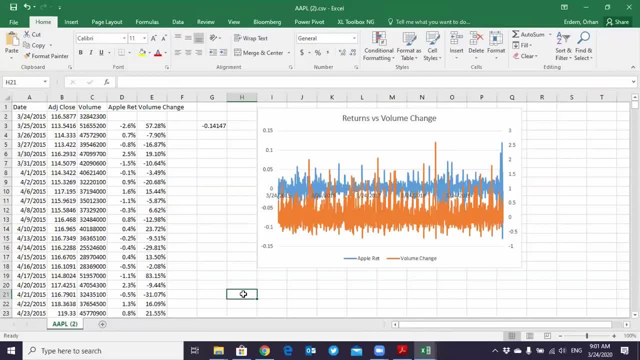 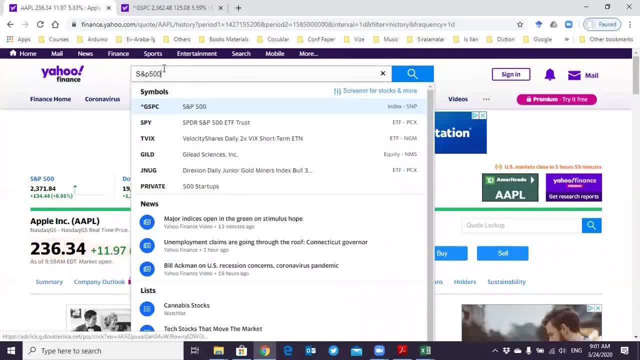 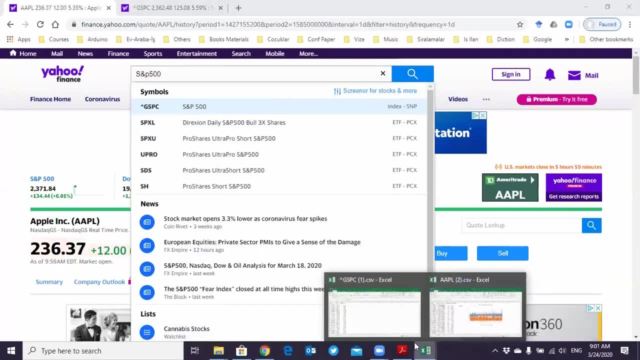 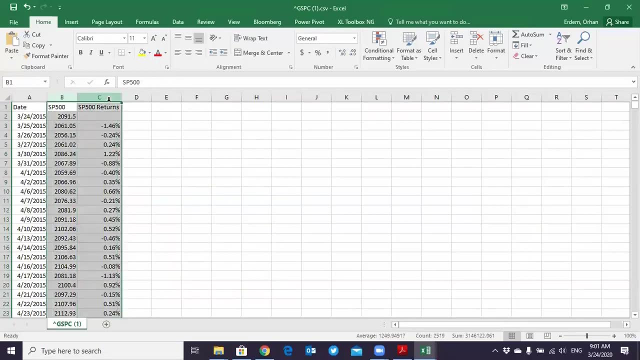 S&P 500 and then do the same thing with this ticker and then download five-year stock price indexes, which I did before I record this video. so it's here. I'm going to copy and paste it to the other Excel sheet. okay, just to save time. so I'm 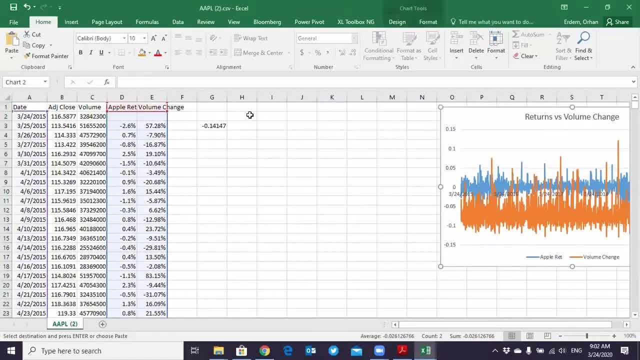 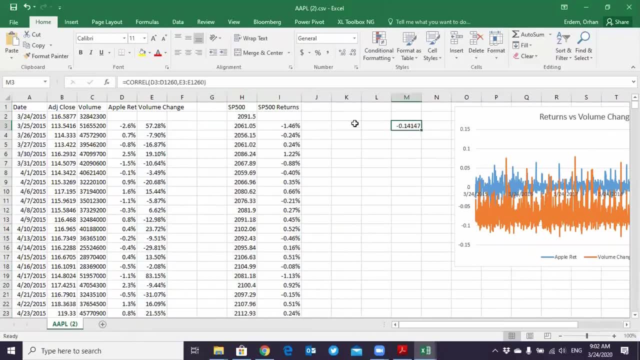 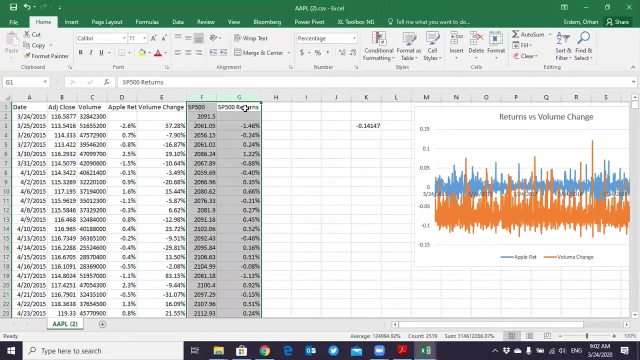 caught. I copied it and I'm going to paste it here. maybe I can just like copy this correlation to here and delete these two columns. so we have S&P 500, S&P 500 returns. so generally when we say market index or market returns, we mean 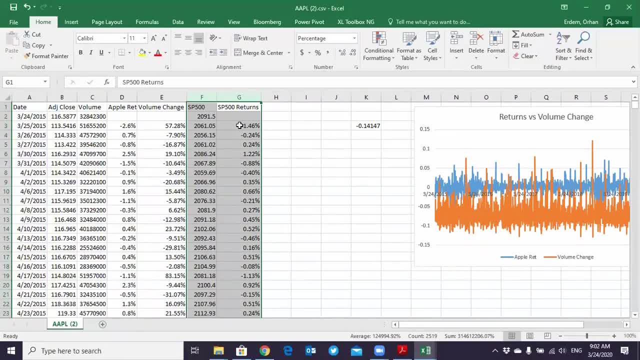 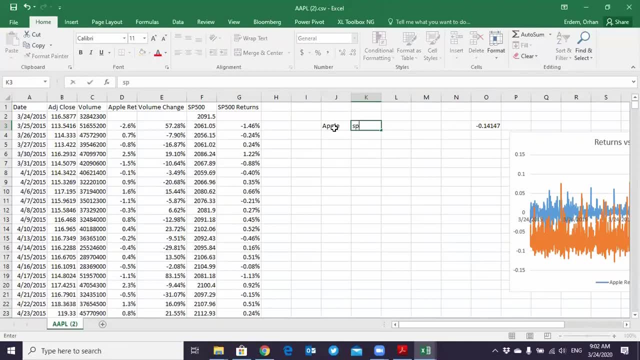 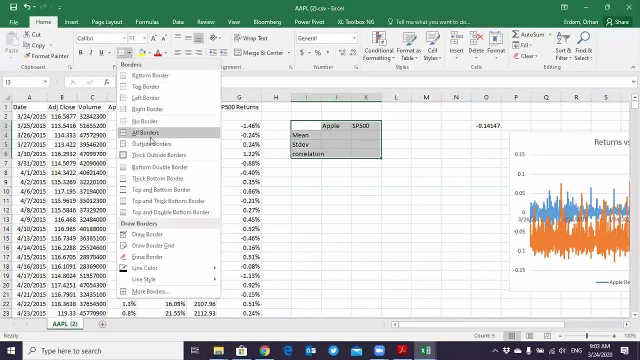 like these indices, market indices, S&P 500. let's compare the performances of Apple and S&P 500. so to do this, right here, Apple, right here S&P 500, just to prepare a table. so mean standard deviation and correlation. okay, so just to do like that. and then now let's compare their performances. okay, hit the very first cell of Apple, mean. 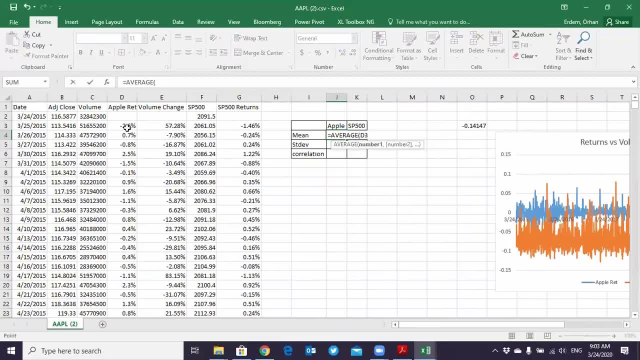 right here average and let's see the Apple returns average. this is Apple return, the same thing for S&P 500 returns. right average and select all column, close the parenthesis. so, just So, let's increase these decimals to two. As you can see, Apple is far higher than S&P 500.. 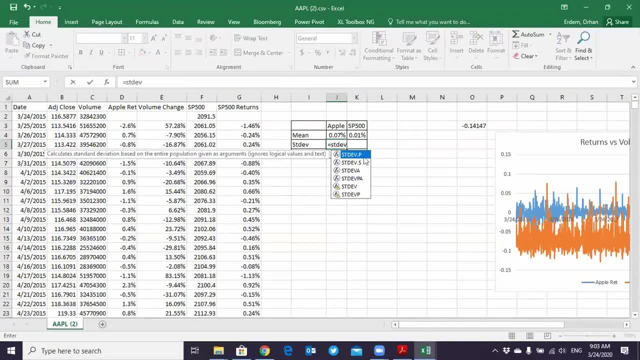 And then do the same thing for standard deviation, STDEV this one And select standard deviation of Apple and then, close the parenthesis, Do the same thing for S&P 500. So basically we are comparing the return performance, average return performance and standard deviation. 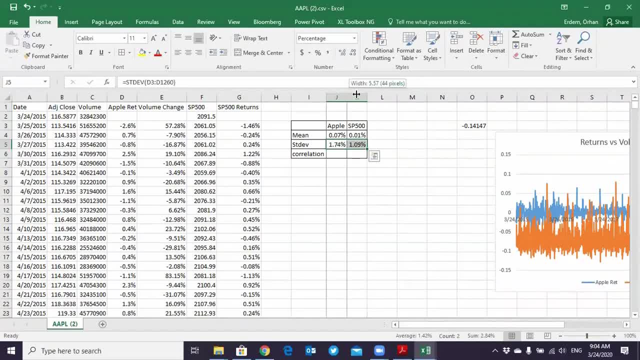 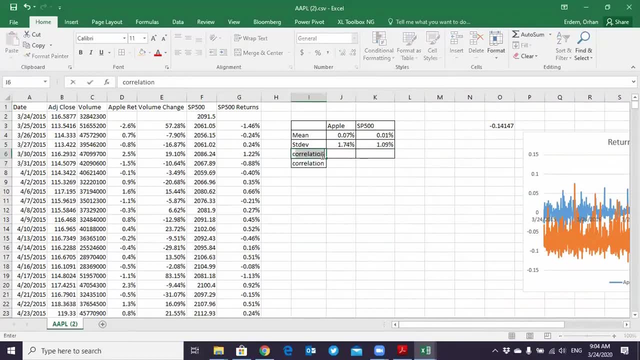 performance of the market indices and stock. So for correlation, I'm going to cut it and paste it here. Let's write here: coefficient of variation- CV. As you might remember, coefficient of variation adjusts the average performance of stock with risk. To calculate coefficient of variation. 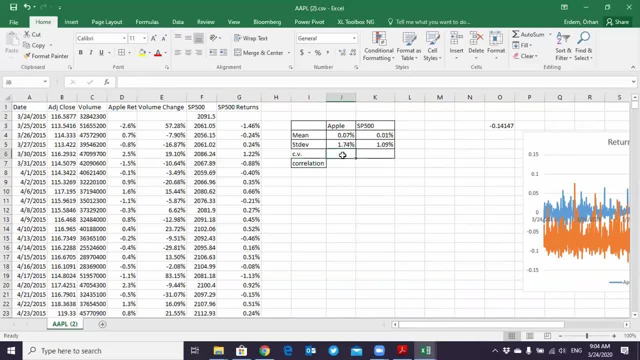 we need to divide standard deviation by the mean, So standard deviation, So let's talk in a minute about this mean and standard deviation. As you can see, Apple is six times higher than S&P 500. mean for a little increase in the risk. 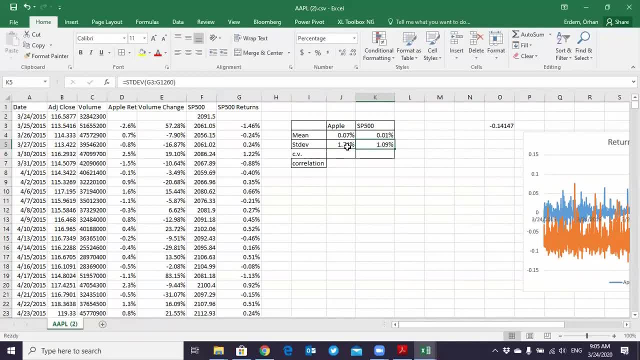 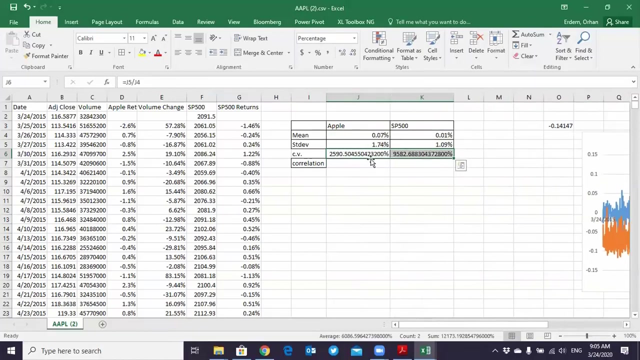 So the risk of Apple is of course, higher than S&P 500. But it gives you only six times higher return. So coefficient of variation is standard deviation divided by average return. Do the same thing here. OK, Let's decrease those numbers to two. 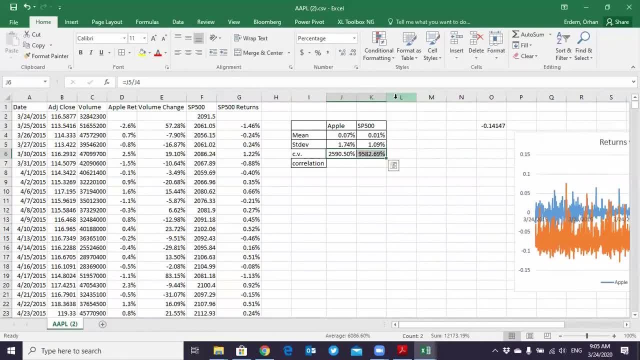 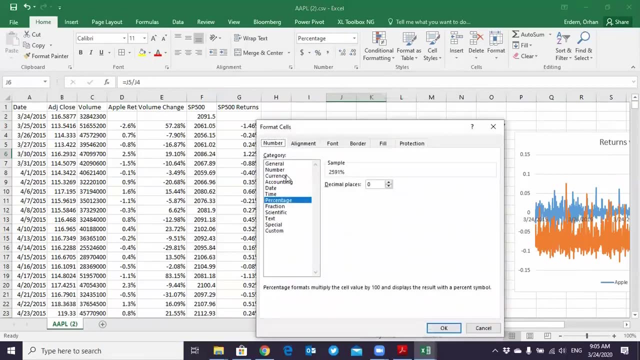 So now you see, it's clearer now that Apple's risk, adjusted by the mean, is like: let's change it to normal numbers, without decimals, without percentages, I'm sorry. So you don't need percentages for decimals. Fine, I mean you can do it. 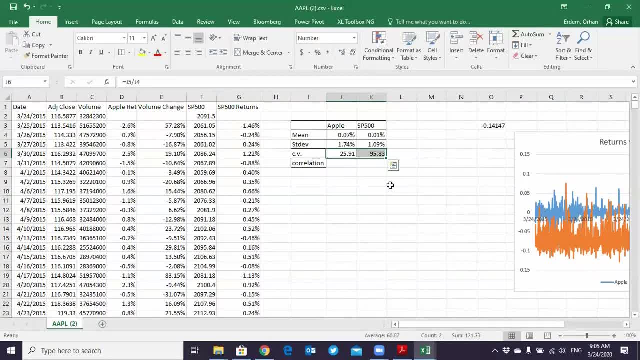 But without percentage, fine. So coefficient of variation of Apple is 25.. Coefficient of variation of S&P 500 is 95, which means that the risk adjusted by return is far higher in S&P 500 than in Apple. So, Apple comparing and just looking at those two variables, 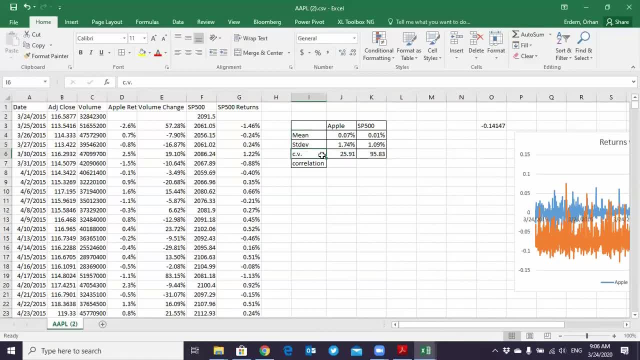 mean and standard deviation. coefficient of variation, which is risk adjusted by mean, is far, so Apple looks far safer than S&P 500.. In terms of those two decimals, those two parameters, This is a simple comparison. Once again, let me summarize before proceeding. 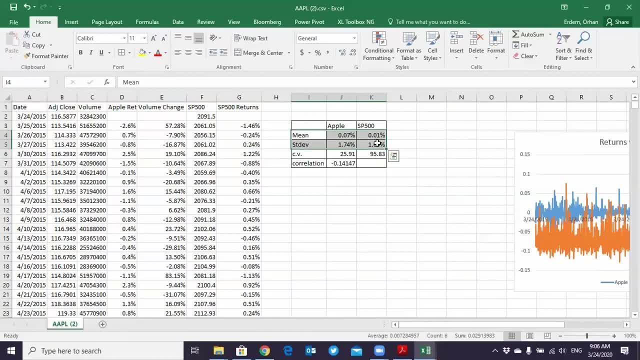 Apple's mean is higher, Apple's standard deviation is higher, But when we use coefficient of variation, adjusting those two parameters, Apple looks far safer than S&P 500 investment. OK, So how about the five-year performance? So let's write here: five-year performance. 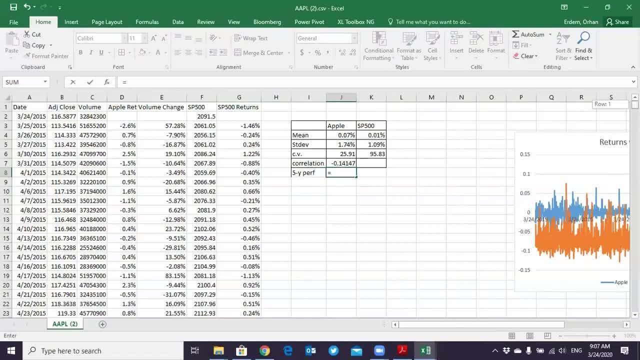 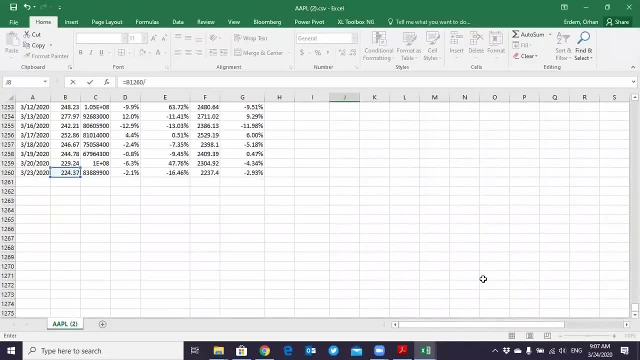 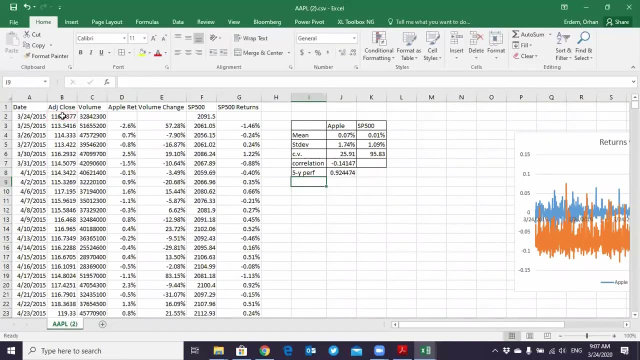 So to do this, let's write here five-year performance. Let's see how Apple performed in five years. So this is Apple's stock prices. So today divided by the day in five years ago. So this is Apple's performance, five-year performance. 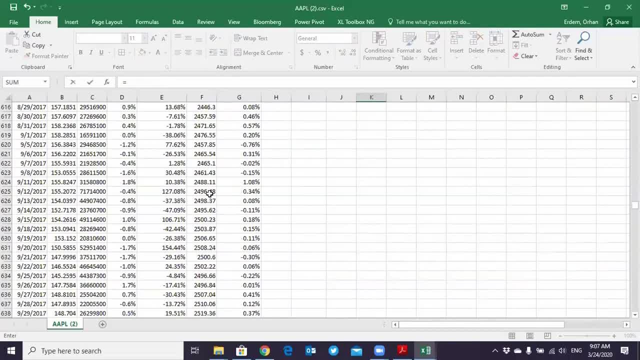 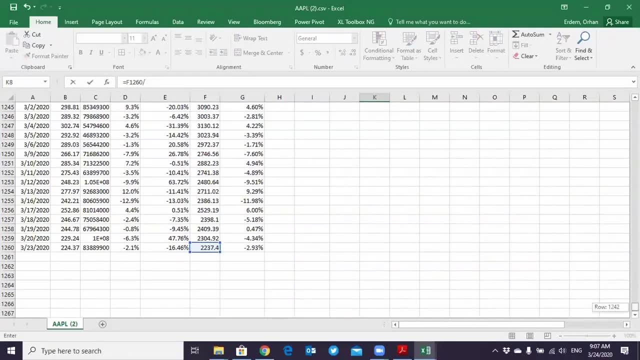 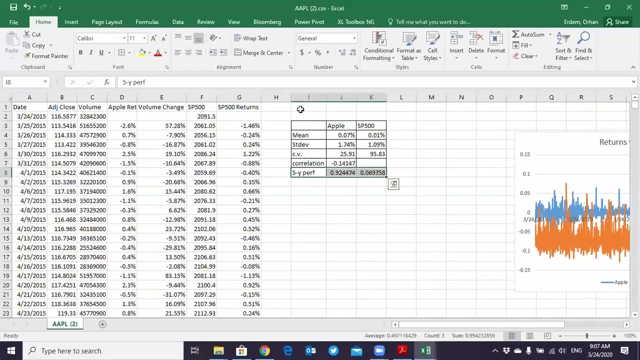 Do the same thing for S&P 500.. Column F is S&P's indexes Today divided by S&P 500. Today divided by the day five years ago. So this is their performance. So in five years Apple's return percentage returns 92%. 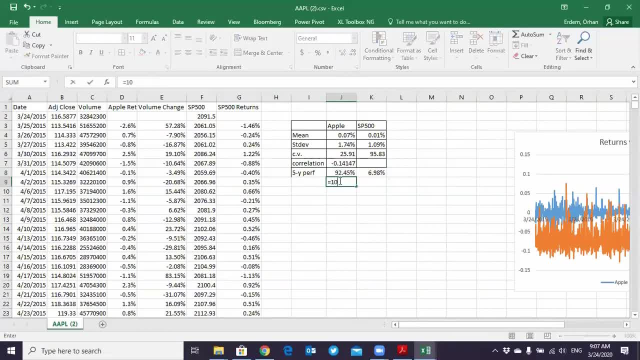 S&P 500 is just 6%. So if you invested $1,000 in Apple, so you would have made $1,924.. If you just like to do the same thing for S&P 500 index, it will $1,069..